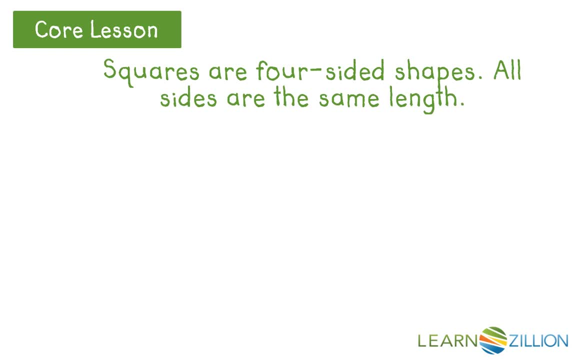 Remember that squares are four-sided shapes and we remember that all the sides are the same length. Here I have a picture of a square. Here I have a picture of a square. Here I have four toothpicks. I notice that the toothpicks 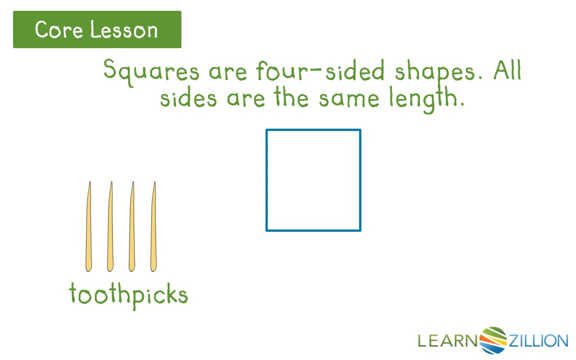 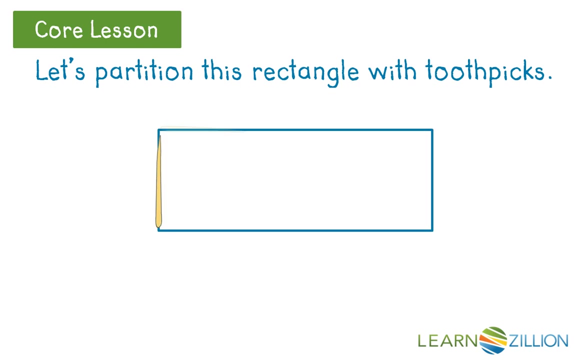 are also the same length. If I place the toothpicks on top of the square, making sure that I am creating square corners, I notice that I can use the toothpicks to form a square. Let's partition this rectangle with toothpicks. I place my toothpicks. 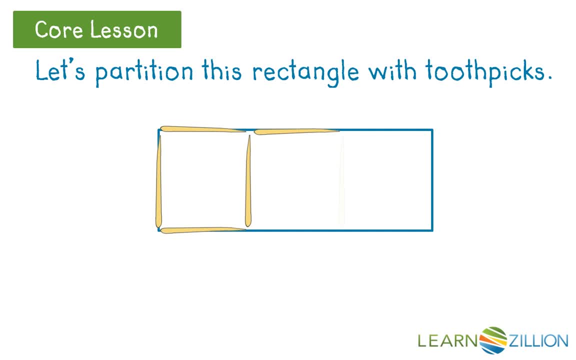 and I make sure that I have created square corners, I make sure that I cover all of the rectangle and I keep adding squares, using the toothpicks to fill the entire rectangle. I notice that I have created one row of squares and I count them: One, two, three. 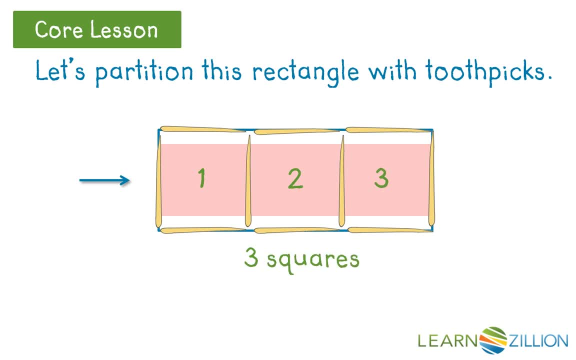 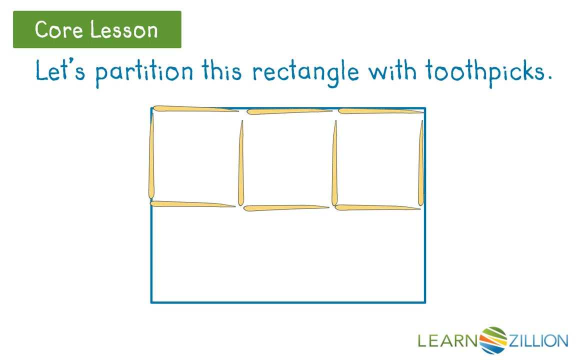 I have created three same sized squares. Here I have a larger rectangle. Once again, I use my toothpicks to form squares, making sure that I create square corners. I have completed the first row, so now I start adding toothpicks to create a second row. 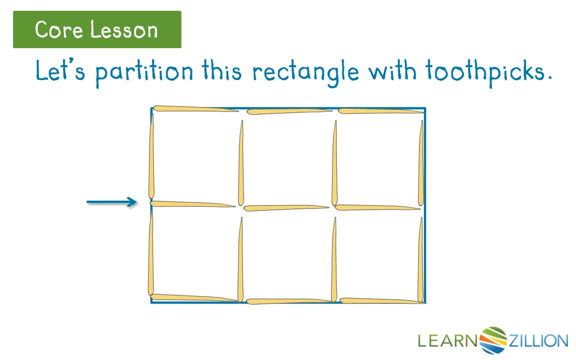 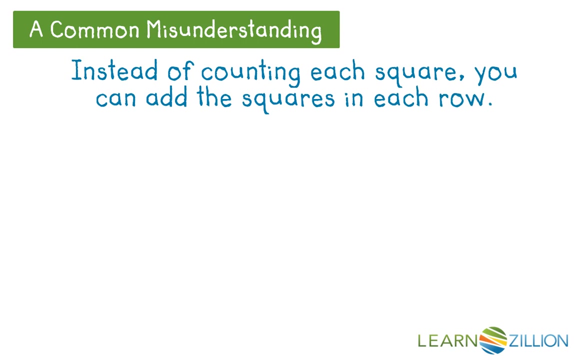 of toothpicks, So I have ended up with two rows. I count the number of squares: One, two, three, four, five, six. I have six squares. Instead of counting each individual square, we can add the squares in each row. 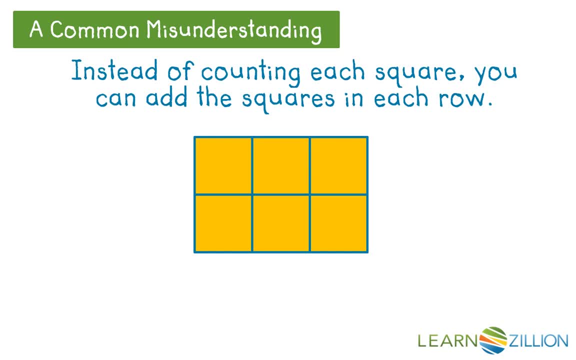 Here I have a rectangle. I notice that it has been partitioned into squares. I count them: One, two, three, four, five, six. This is one way of figuring out how many squares in our round can be out, how many squares are inside the rectangle. Instead, I can take a look at